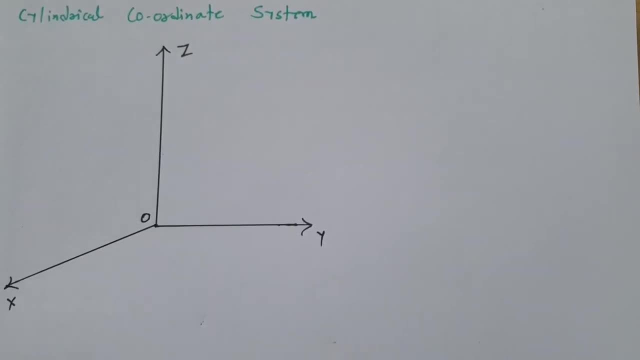 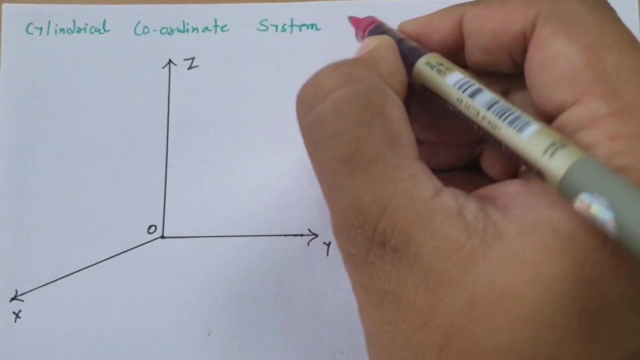 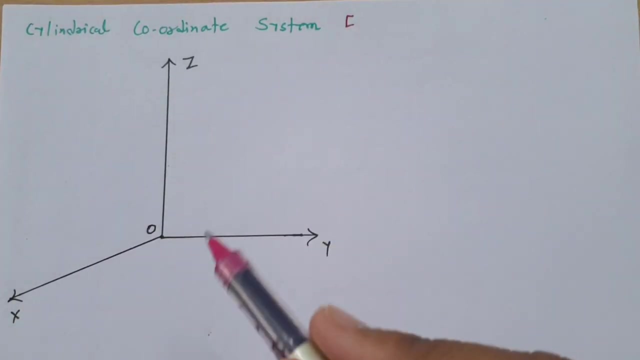 Welcome to Electromagnetics Playlist I. Professor Itesh Dholakia is going to explain you cylindrical coordinate system in this session. Now, see, I will be explaining cylindrical coordinate system in comparison with Cartesian coordinate system, where we have already seen Cartesian coordinate system and that we are explaining with respect to x-axis, y-axis and z-axis right. 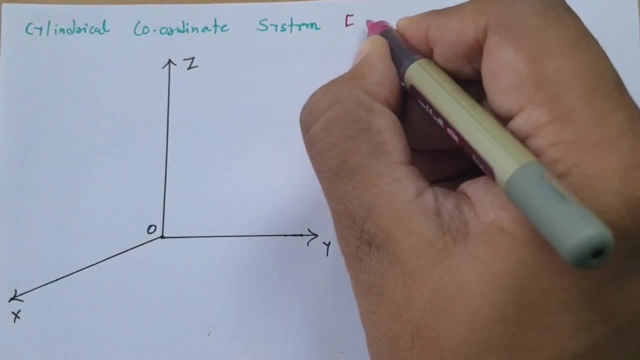 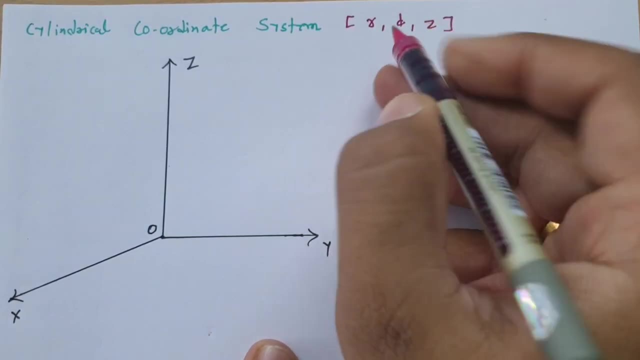 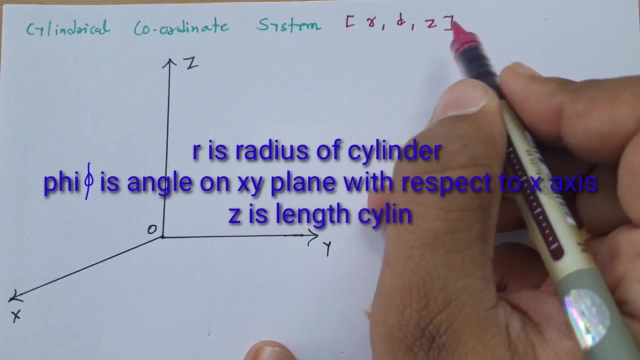 So in cylindrical coordinate system we have three coordinates and that we represent by having r, phi and z. So these are the components: r stands for radius, phi is angle with respect to x-axis on x-y plane and z is length of cylinder. 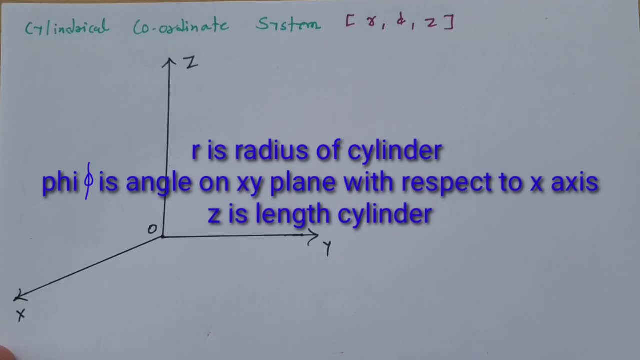 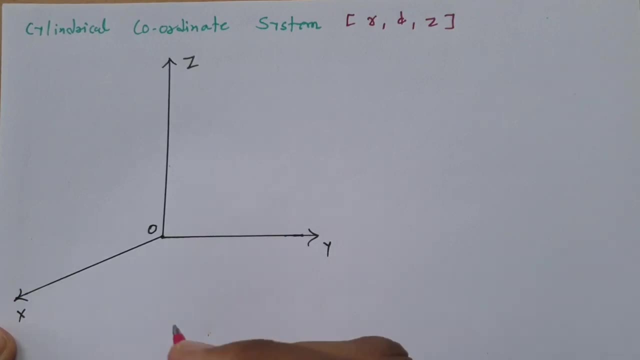 That is what we are delivered to understand in this session. Now let us try to understand that with respect to one point first, So it will be clear to all like how we can assign any Point in cylindrical coordinate system. So see, if I say I have one point and that is over here, and let us say this point is x, y, z point. 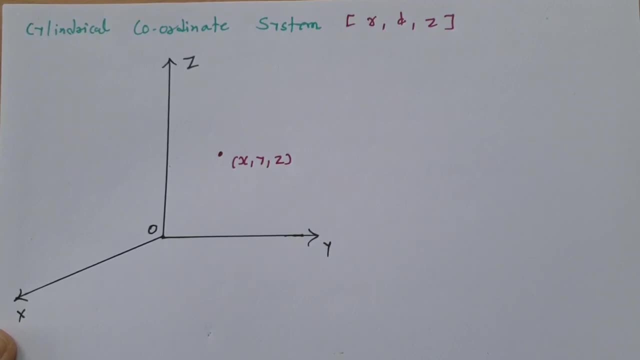 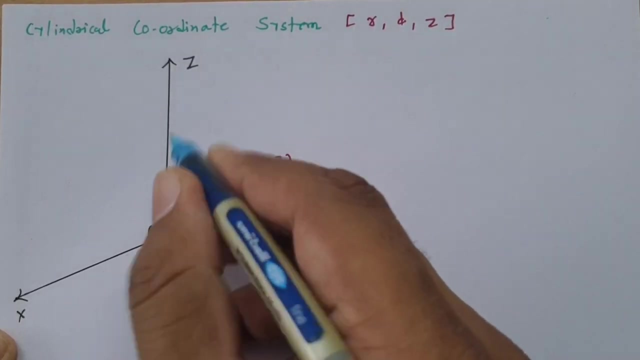 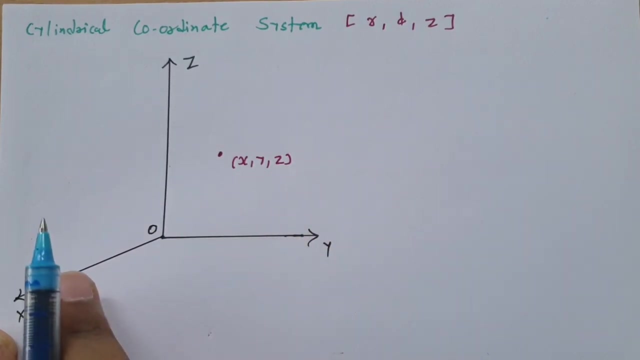 Now how to assign that in cylindrical coordinate system. So for that I will be drawing one quarter cylinder over here and that quarter cylinder that is there in plus x to plus y direction with respect to z. So length of cylinder, length of quarter cylinder that is there with respect to z-axis, and that quarter part of cylinder that is there in positive x and positive y. 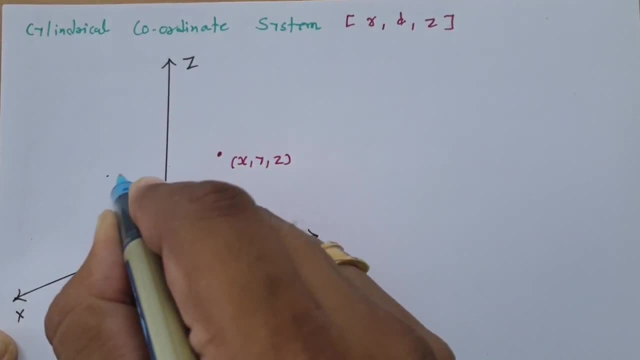 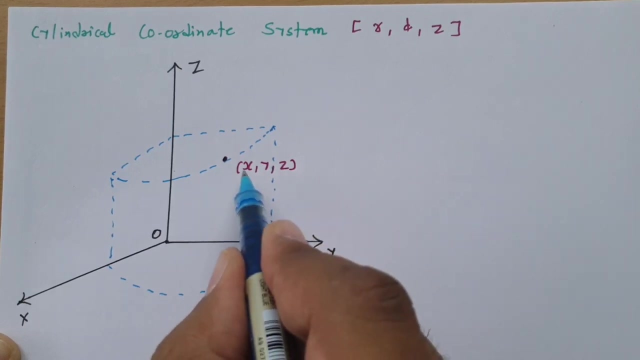 So let us draw it first So you can see where projection of this point on x-y plane. if I stretch it, then that will be coming over here right Now. see, let us try to understand what is r, what is phi and what is z. 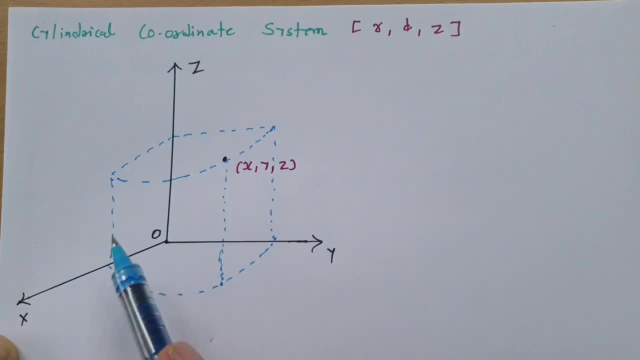 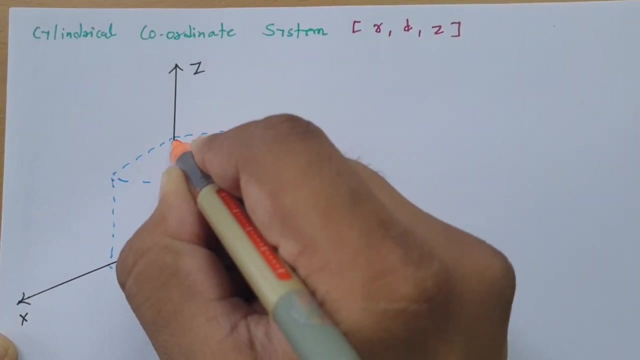 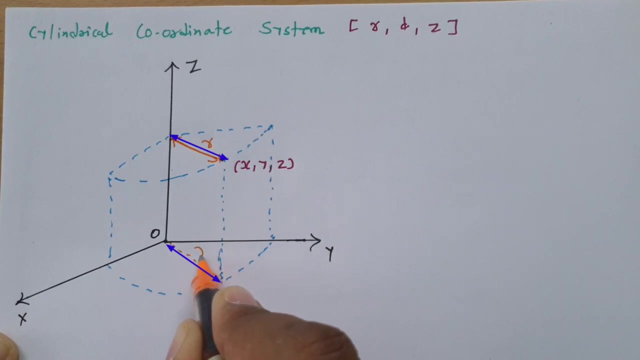 See, r is radius of cylinder with respect to x-y plane over here, right? So if you want to show what is the radius over here, then see, this is what A radius. So this distance is a radius And even if you see this trajectory, this distance is even. 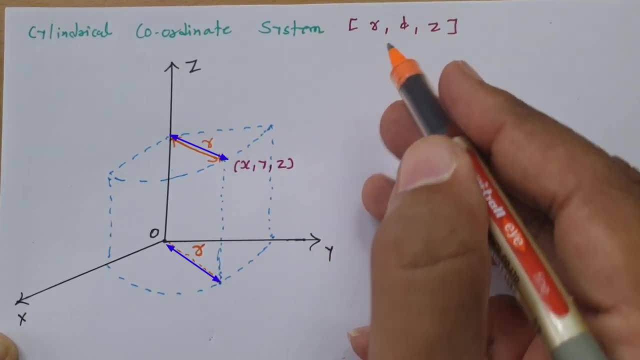 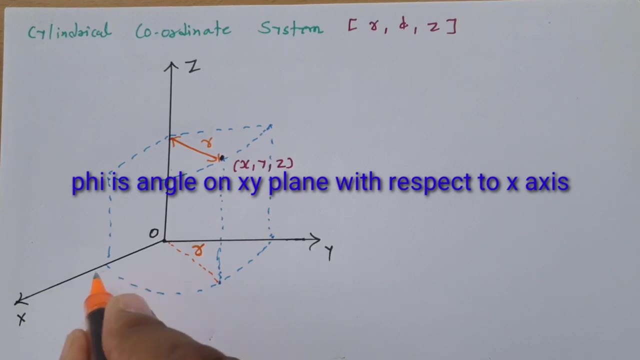 So this is what A radius r. Now, what is phi? So phi is angle on x-y plane with respect to x-axis. So see, this is what x-y plane and this is phi, which is what angle with respect to x-axis on x-y plane. 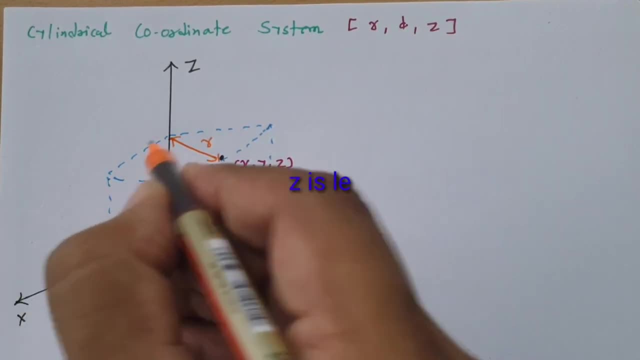 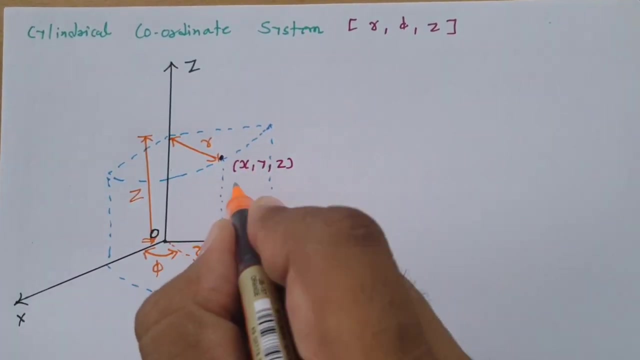 And what is z? z is length of cylinder. So if you observe this is what the length which is there with this cylinder. So this is z, So we can see that this is z. So we can say, in cylindrical coordinate system these coordinates are r, phi and z. 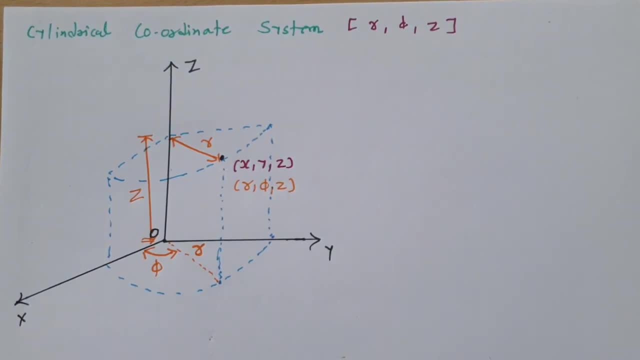 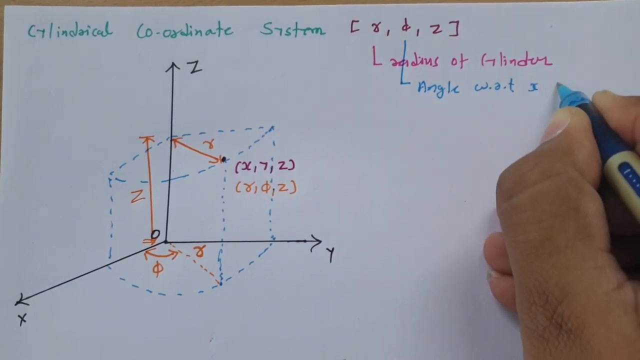 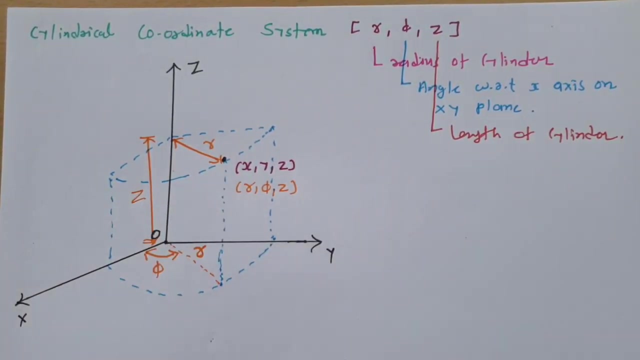 So let me mention that one by one. See, r is radius, phi, that is angle with respect to x axis, One xy plane, and z is length of cylinder. So this is what the coordinates which is there with cylindrical coordinate system, and you should know the diagram with respect to all dimensions. 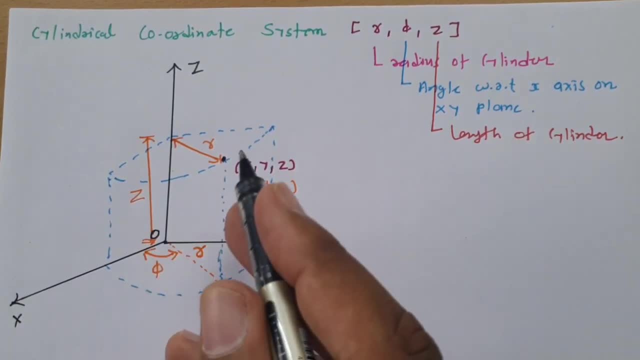 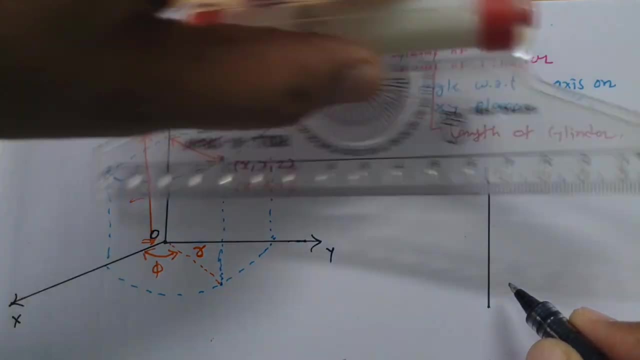 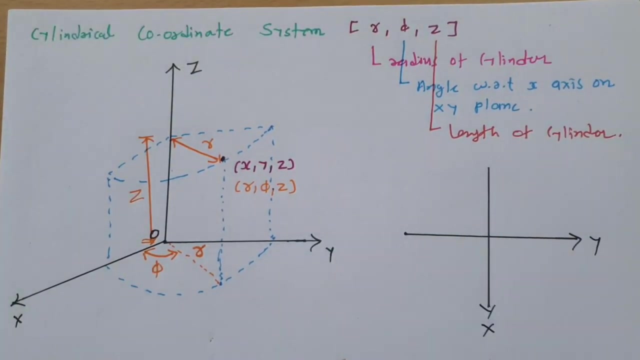 Like, if I talk about top view, how top view will look like for this situation, Then let me draw it over here first. See, this is x axis, this is y axis and I have drawn. see this quarter cylinder, You can see, and in that, if I say: this is what a projection. 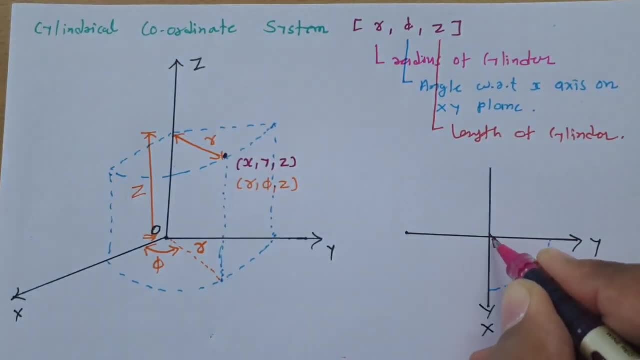 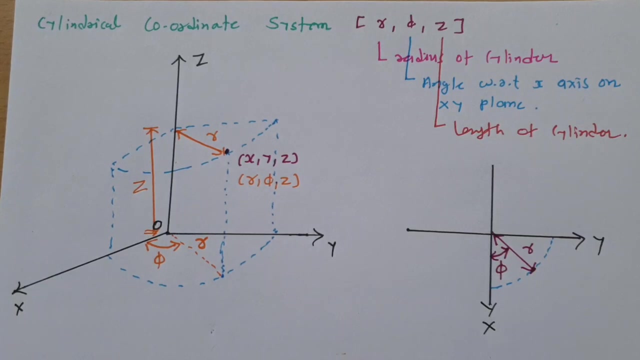 So we can say this radius, that is r, And this angle, that is phi, And length of cylinder, that is z. See, this is how it is there. Now, here I will be going to explain you how to convert cylindrical coordinates into Cartesian coordinates. 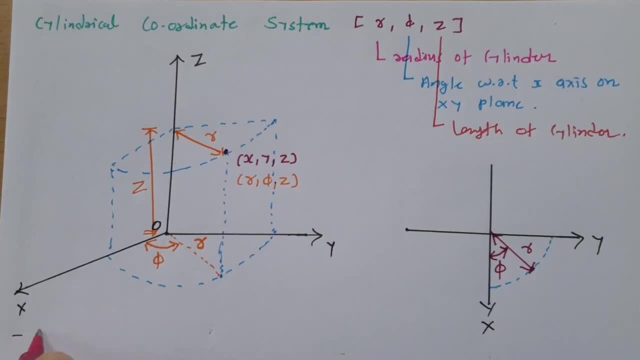 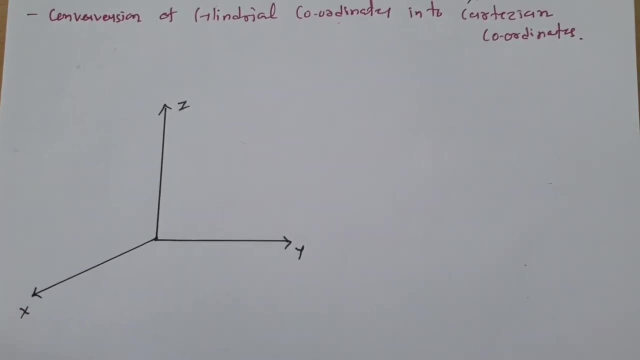 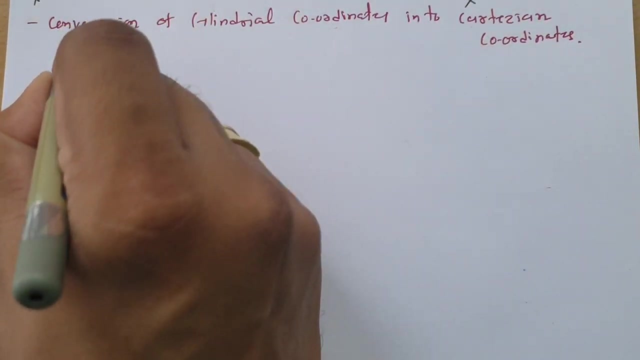 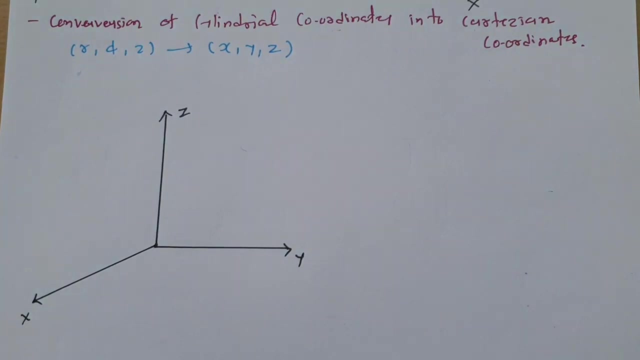 So let us mention that. So let us have cylindrical, Okay, Coordinate conversion into Cartesian coordinate conversion. So our agenda, that is to translate r, phi, z into x, y and z. Now here let us say we have a point and that point is placed here, and that point is r. 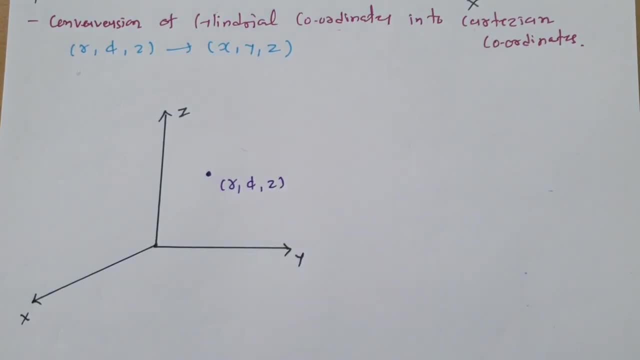 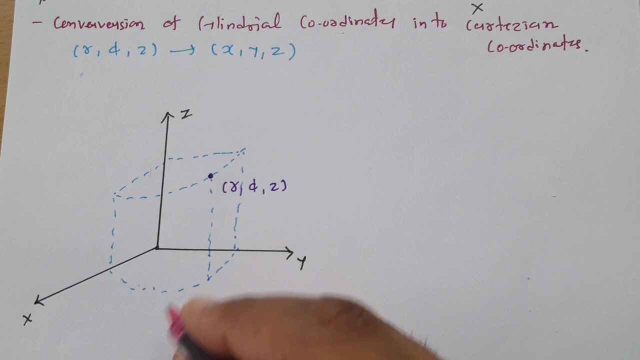 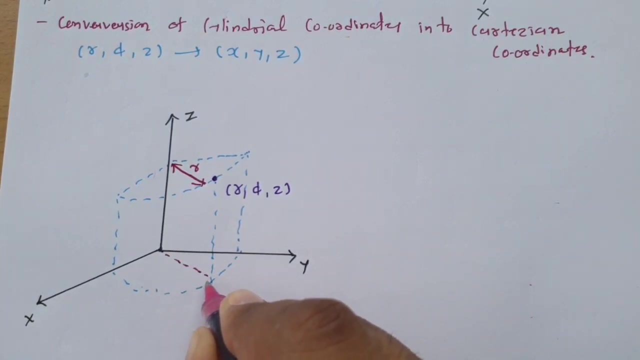 phi z right, So as if I plot quarter cylinder, Then you can see. I am just drawing it right now first. So what is radius in this situation? This is what radius Right And with this trajectory, if I take this angle with respect to x axis, then that angle is: 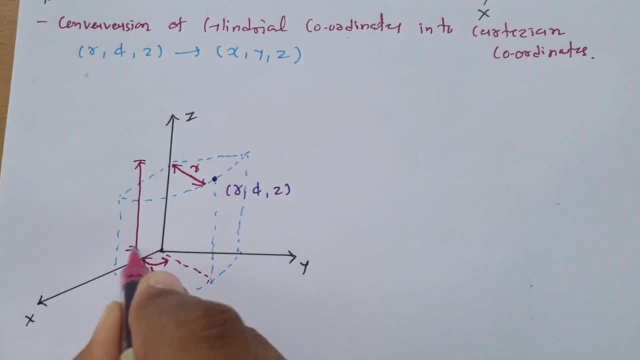 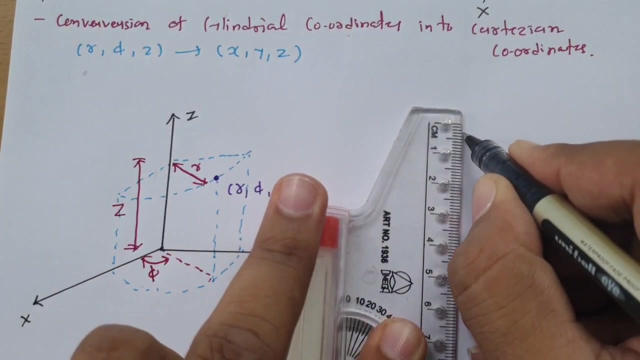 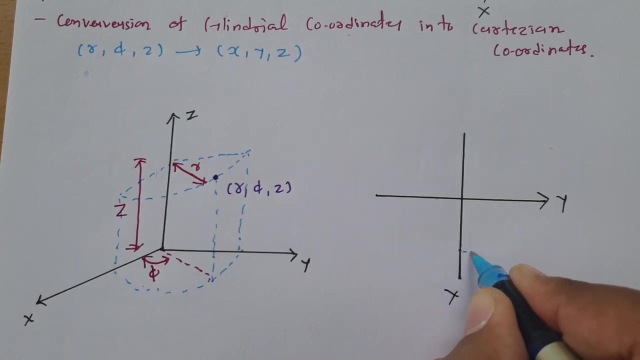 phi And This length of cylinder That is z. So how to convert this into x, y, z. So see for that. let us see top view of the cylinder. So I am just drawing top view over here Now. see, in this top view, if you observe this cylinder- and I have, I have drawn quarter. 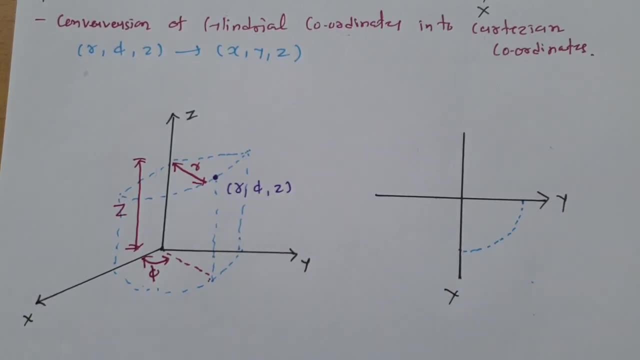 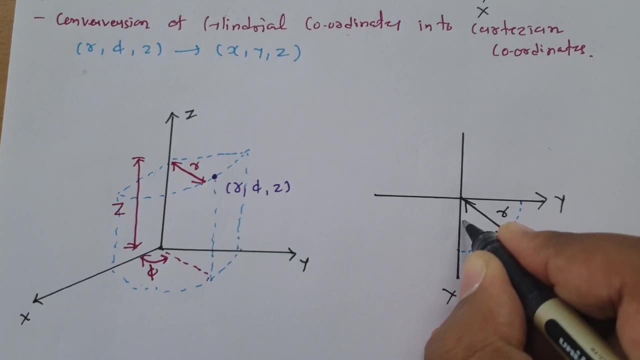 cylinder over here, Right Where, If you see This Point like this, This is radius r and this is angle phi. So how to calculate x, y, z components. So see, this is what radius r And based on radius r, we can calculate x component and y component. 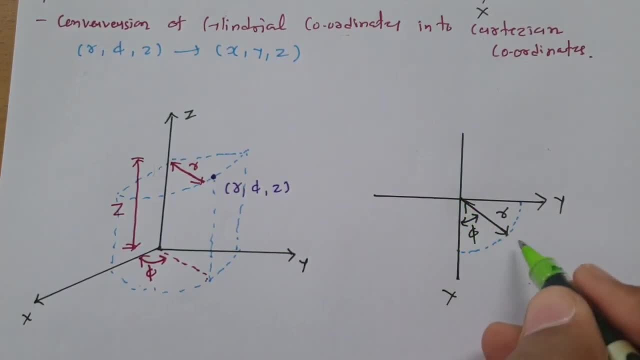 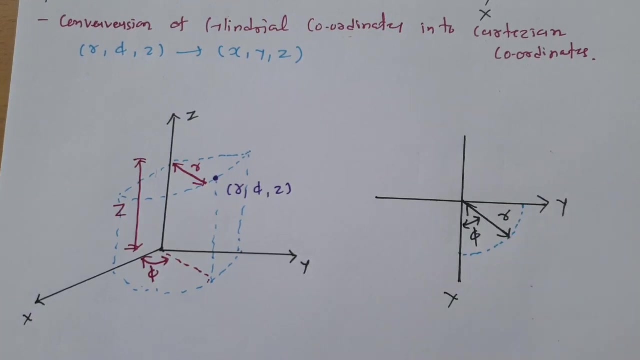 See how to calculate x and y component. So if you observe this triangle, If you observe this triangle, In this triangle, x component is cos component And y component That is sine component, Right? So let me draw it separately See, this is how x component is there. 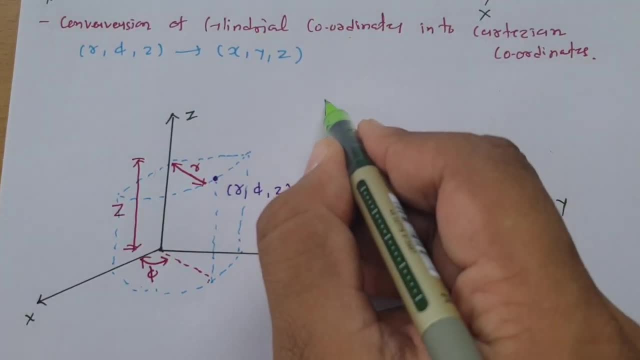 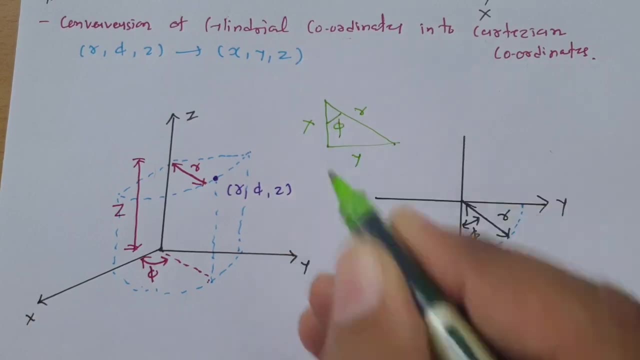 From this triangle. Well, this is radius r, This is x component, This is y component And this is angle Phi. You can see, This is how this triangle is there. So what is x over here? X has to be r cos phi. 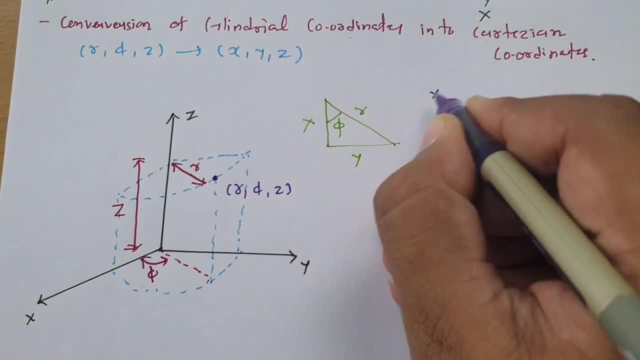 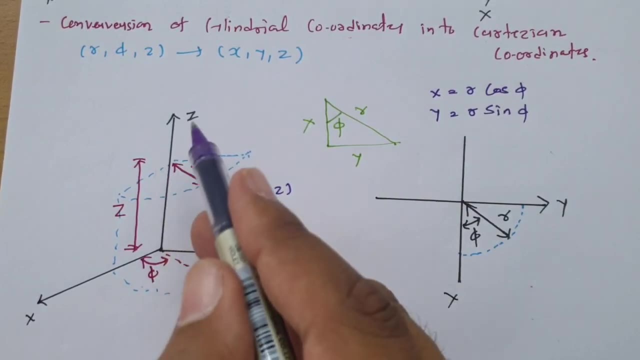 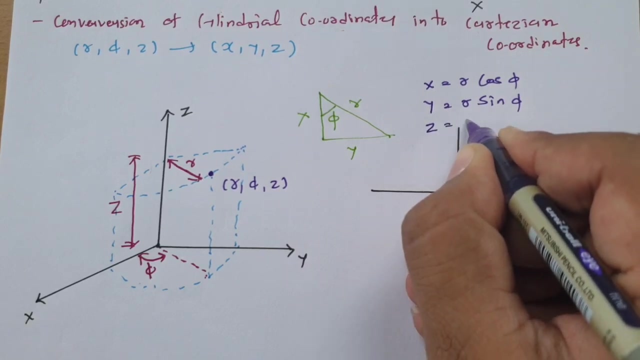 And y has to be r sine phi. So x is r cos phi, Y is r sine phi. And if you observe length of cylinder, So z component is similar in both Cartesian as well as cylindrical. So z is equals to z. See, this is how. 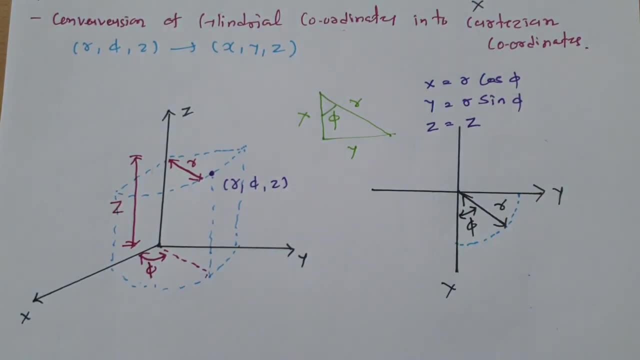 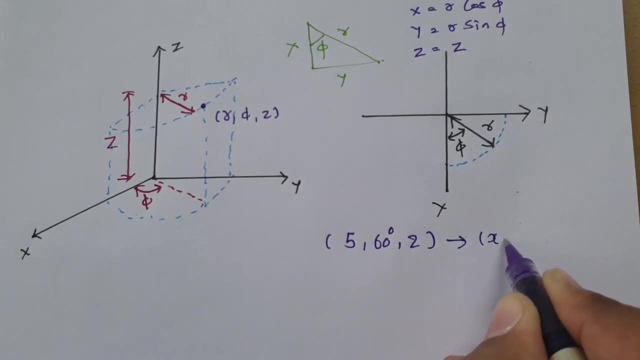 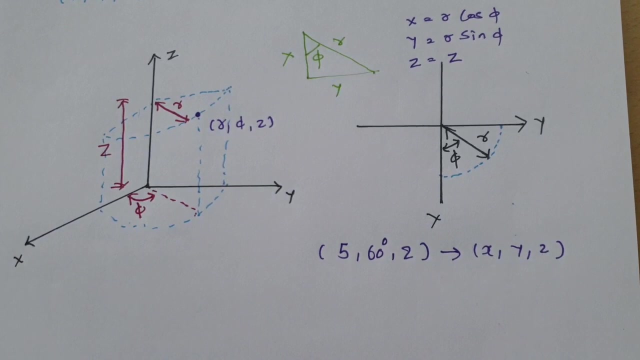 See, this is how we can translate, So let us have one example, So it will be bit more. Convert this point into x, y, z Cartesian coordinates. Then we need to use these three formula, as we have discussed earlier. So x component over here. 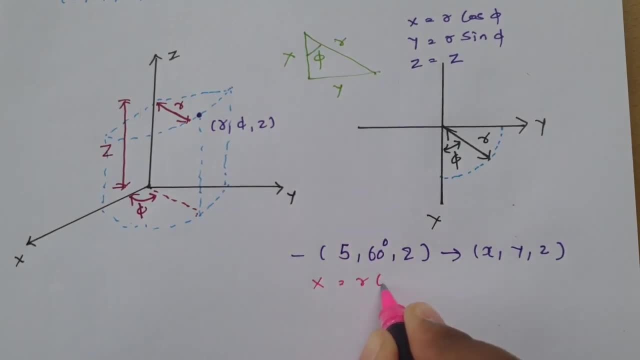 X component, that is r, cos phi, What, where? r is how much Phi And cos phi. Phi is 60. So phi cos 60. And cos 60, that is half. So this will be phi by 2. Here y will be r sine phi. 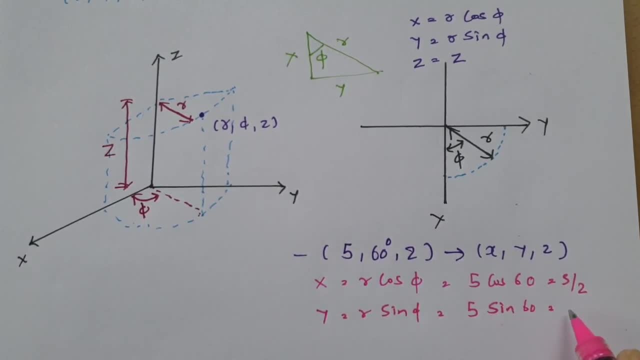 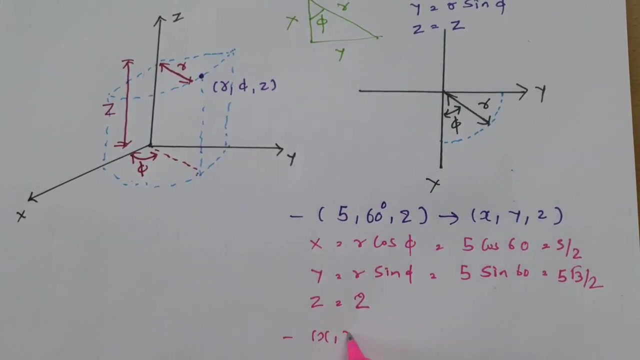 So phi sine 60. Sine 60 is root 3 by 2.. So phi root 3 by 2.. R is phi And z is equals to 2, only Right, Right. So this is how we can translate here: x, y, z, that is phi by 2, phi root 3 by 2 and 2.. 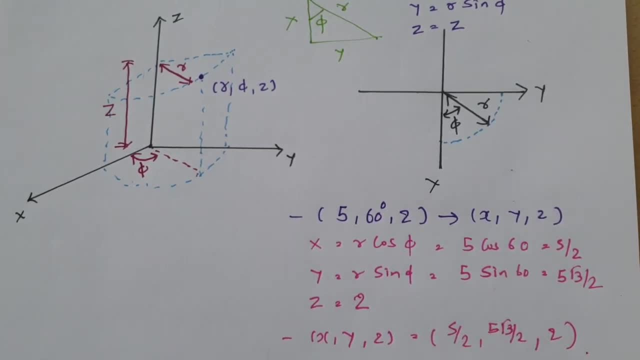 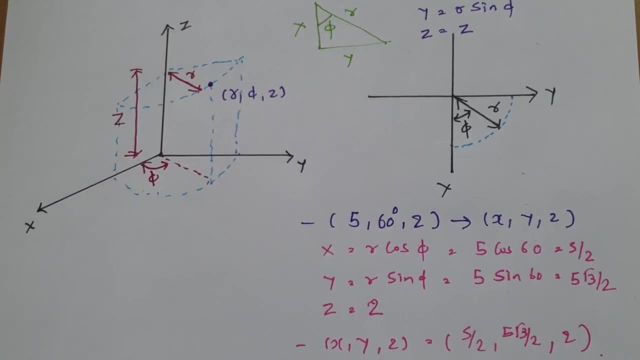 So this is how we can convert this cylindrical coordinate point into Cartesian coordinate point. Now I will explain you how to convert Cartesian coordinate point into cylindrical coordinate point. So let us try to understand that. So to understand that, first of all we need to understand what is radius. 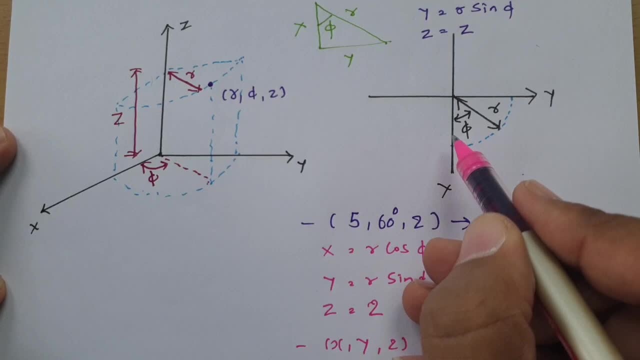 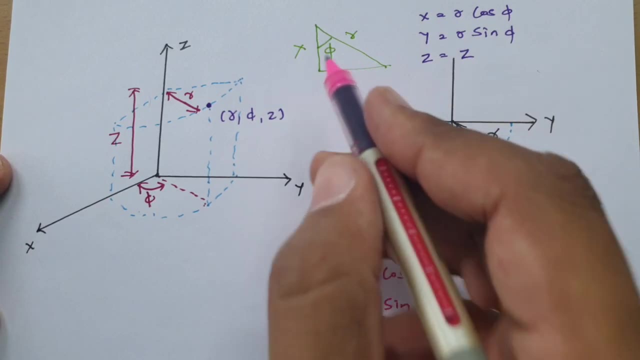 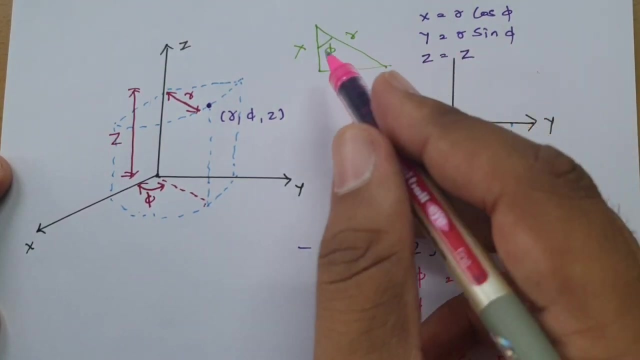 So, as I have told you this, x component is r cos phi and y component is r sine phi, Right. So, based on that, what is radius? Radius based on that will be square root of x square plus y square, And what is angle phi?